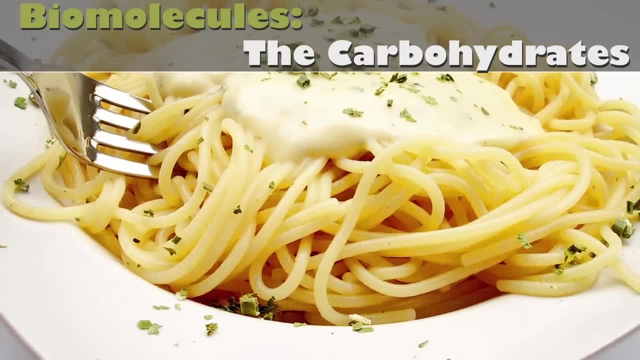 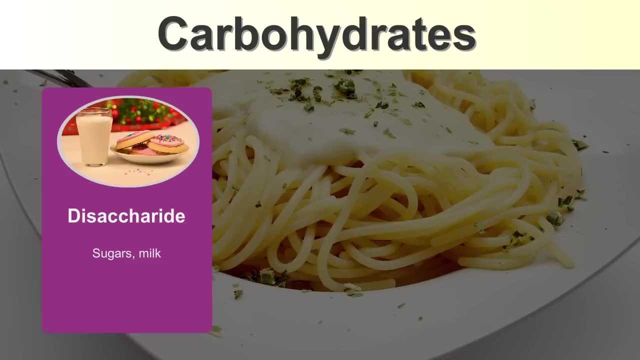 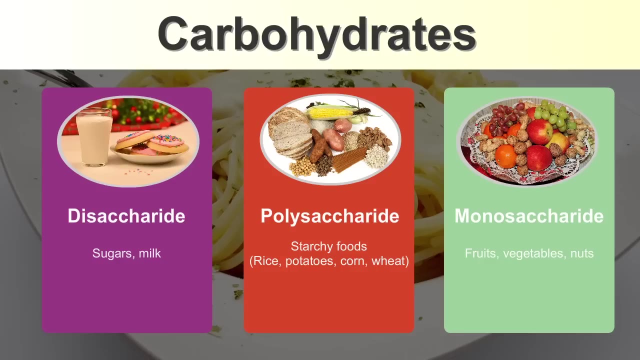 Welcome to The Carbohydrates. In this module you'll explore what carbohydrates are. Carbohydrates are the sugars, starches and fiber found in the foods we eat. They are one of the main nutrients in our diet. Carbohydrates are organic molecules with the general formula: 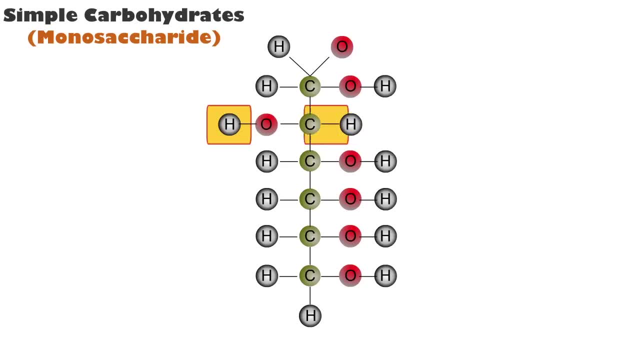 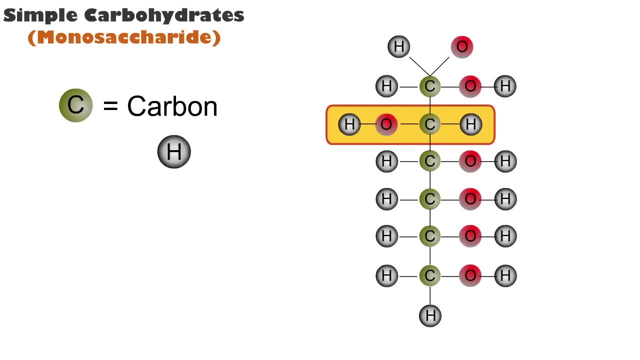 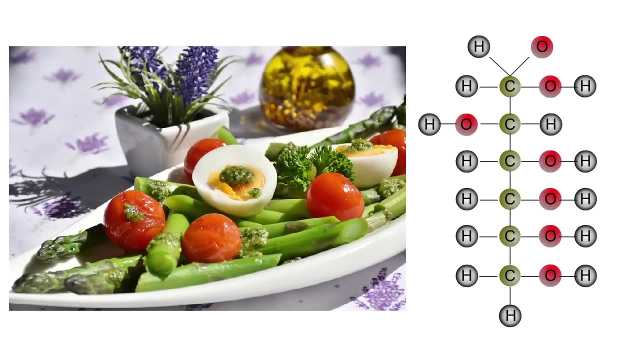 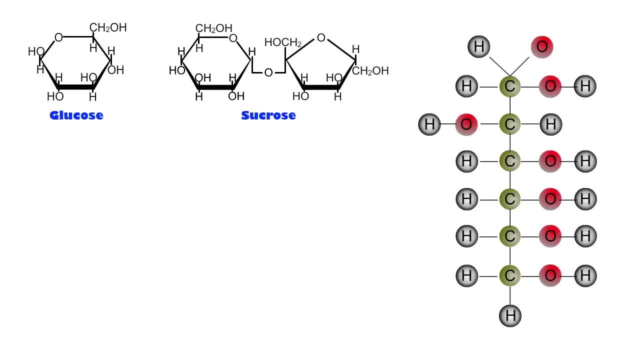 of CHO in a 1 to 2 to 1 ratio. In this formula, C stands for carbon, H for hydrogen and O for oxygen. Although carbohydrates constitute only 1 to 2 percent of cell mass, they provide the raw fuel for cellular energy production. Carbohydrates are classified according to: 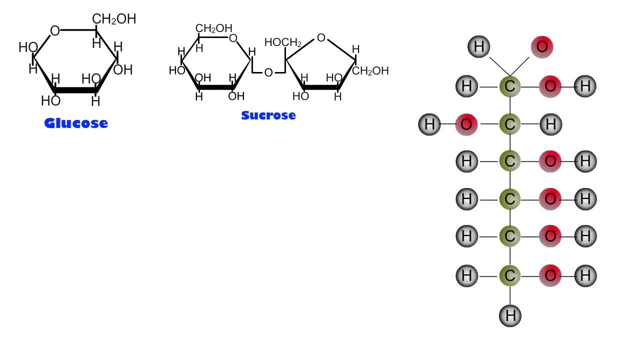 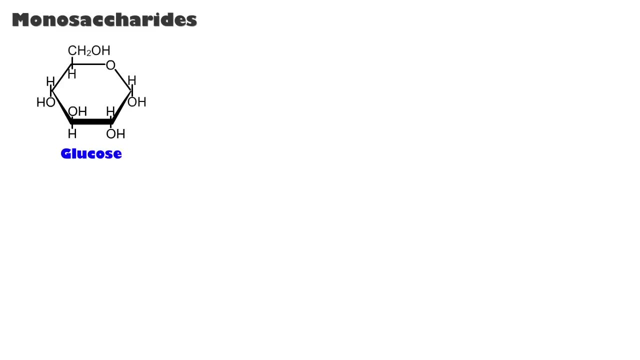 molecular size and solubility. In general, the smaller molecules are more soluble than the larger ones. Monosaccharides include glucose, fructose, galactose, deoxyribose and ribose. Monosaccharides are a single unit. 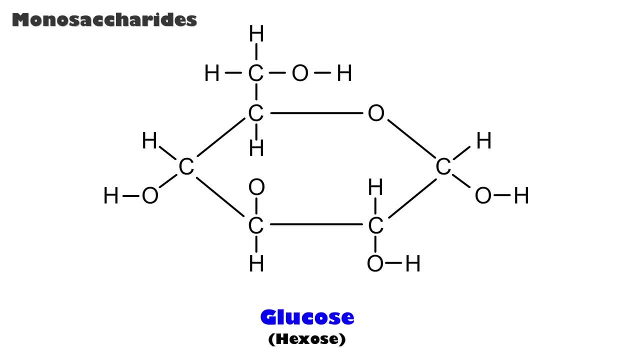 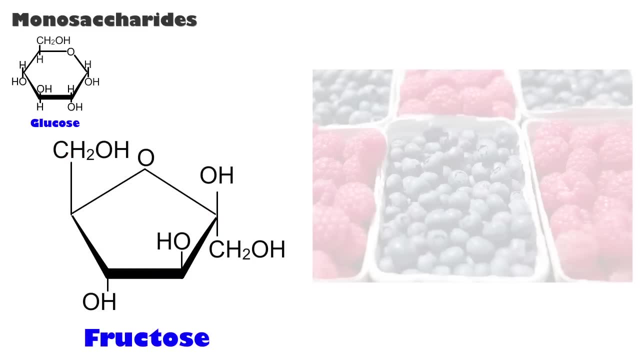 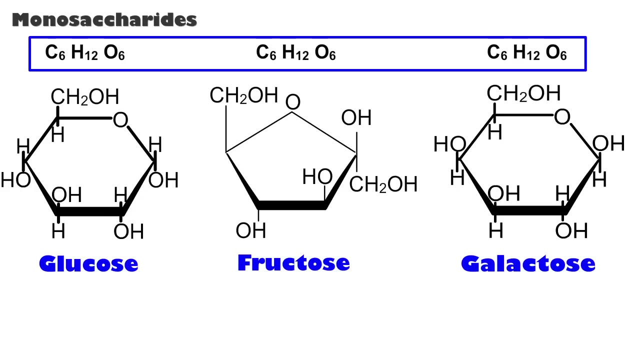 of sugar and are the smallest carbohydrate: Glucose, a six-carbon sugar. hexose is the sugar in our blood. Fructose, the sugar that sweetens fruit. And galactose, the sugar found in milk. have the same chemical formula as glucose and are: 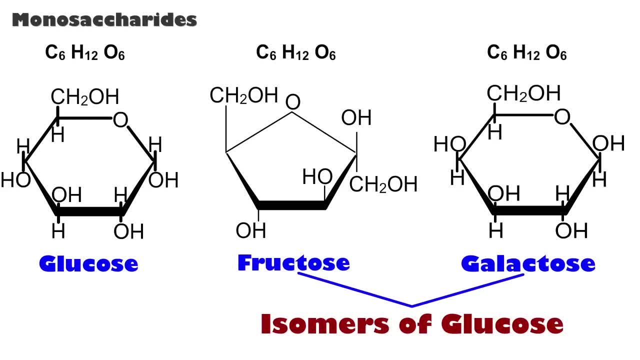 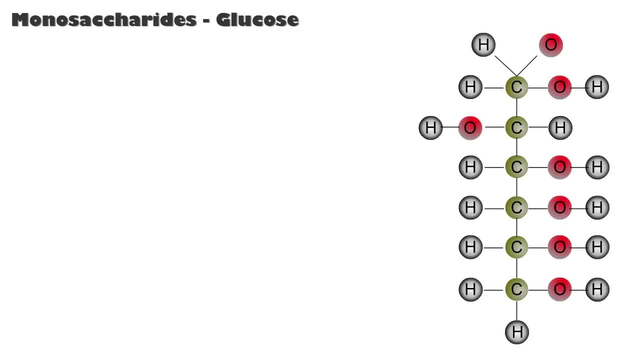 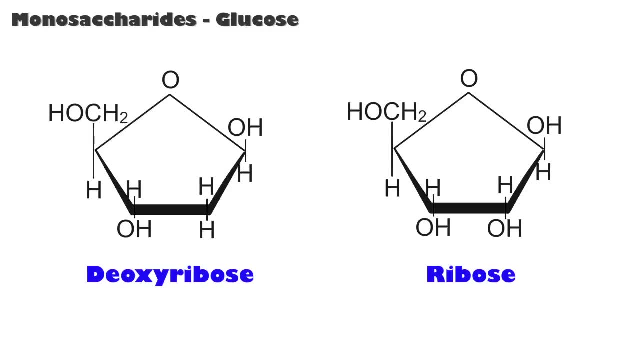 therefore isomers of glucose. Isomers have the same composition but have a different arrangement of their atoms and properties. Glucose can have a straight chain of carbon atoms. However, it's more common to find them in a ring structure. Two other five-carbon sugars, or monosaccharides called pentoboxes, are called pentoboxes. 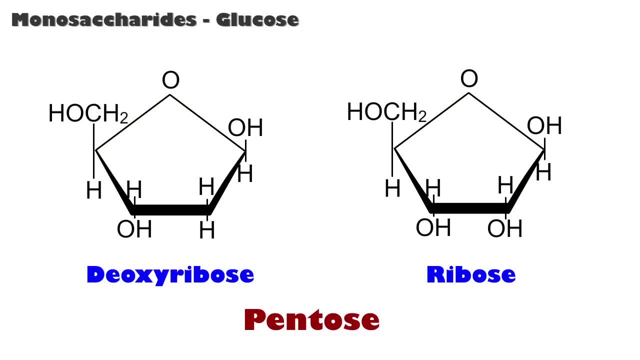 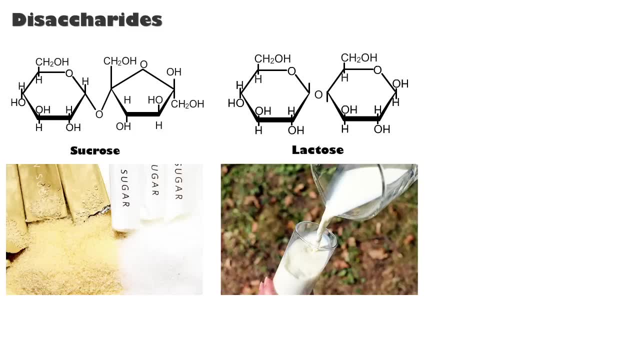 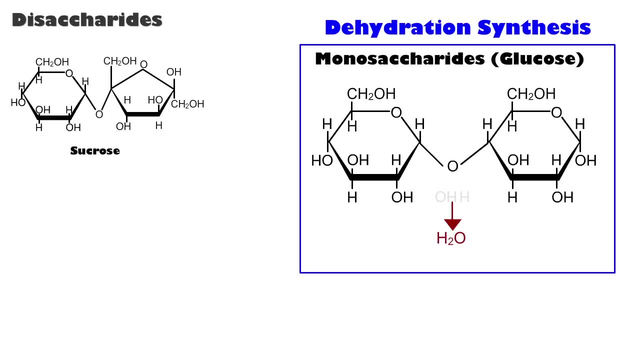 or pentoboxes, or pentoboxes or pentoboxes. The main types of monosaccharides are deoxyribose and ribose. Disaccharides include sucrose, lactose and maltose. Two monosaccharides join together by dehydration synthesis to form a disaccharide molecule.